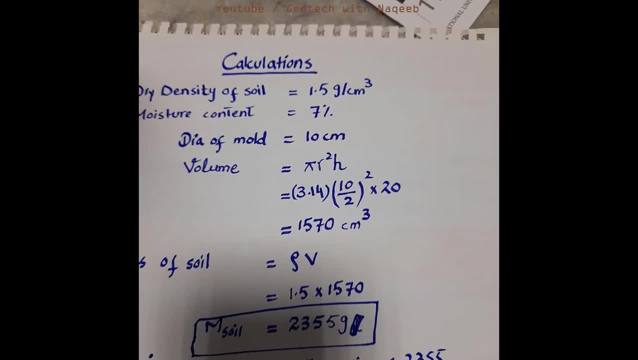 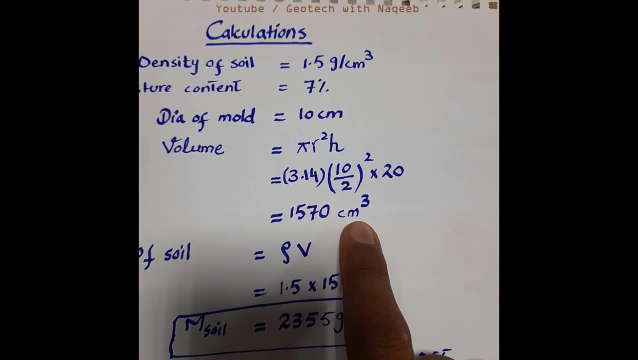 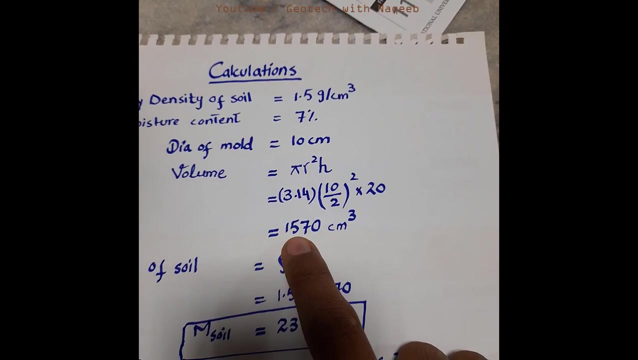 radius, that is, 10 divided by 2 and 20 centimeter, is the height, and the volume comes out to be 1570 centimeter cube. now how will determine the mass of soil required to fill this volume? basically, so, as we know that the formula to find out the mass of soil is density into. volume. so we have the dry density, that is 1.5 gram per centimeter cube. we'll multiply it by volume, that is 50, 70 cubic centimeter, and the mass of soil comes out to be 2355 gram. now we'll take 2355 gram of soil sample. you can see here: 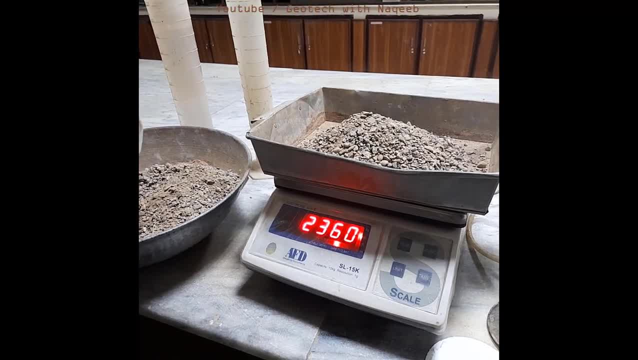 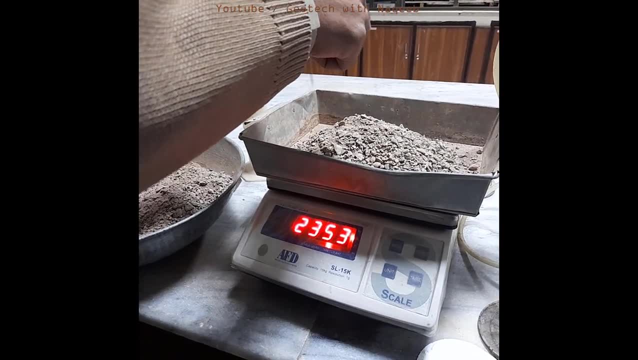 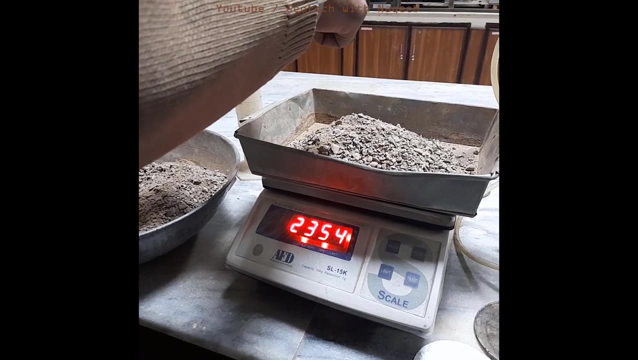 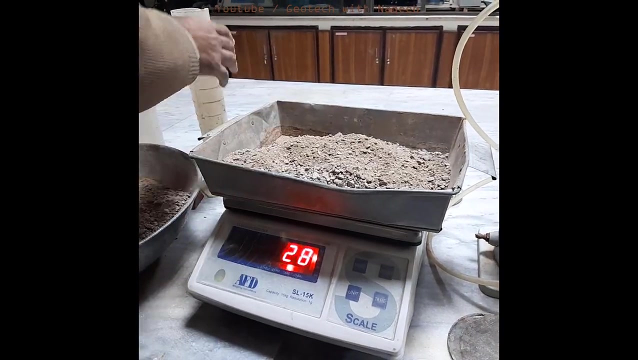 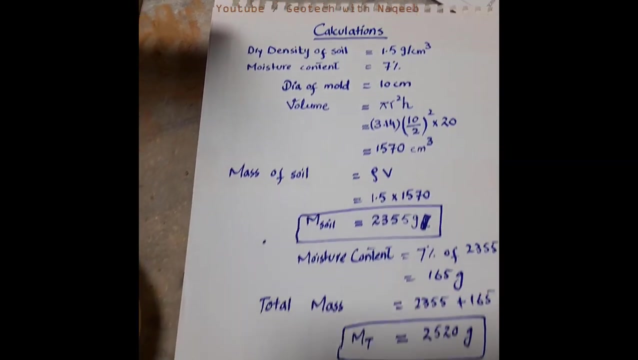 so we have 2355 gram of soil sample. now we need to prepare a remolded sample. we'll have to add some moisture content. how? as you can see here, we have the moisture content. that is 17 percent. so how we'll calculate the moisture content in grams or volume? so it is basically 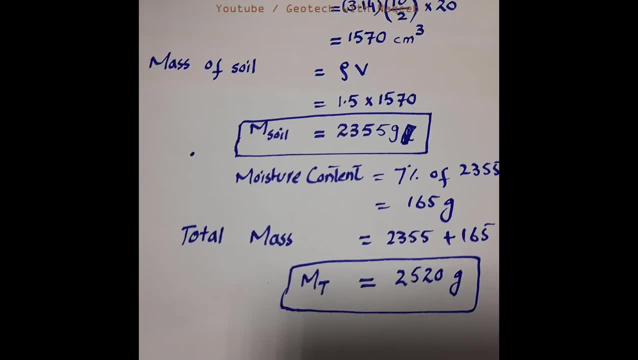 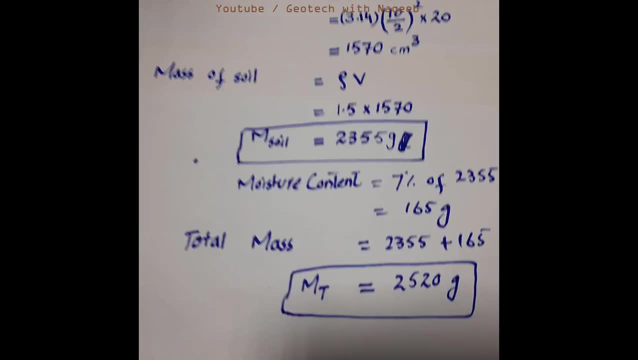 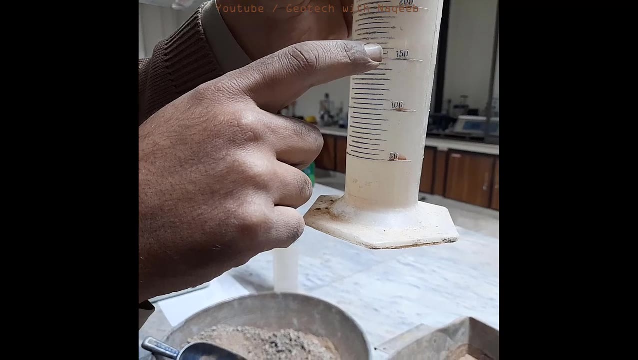 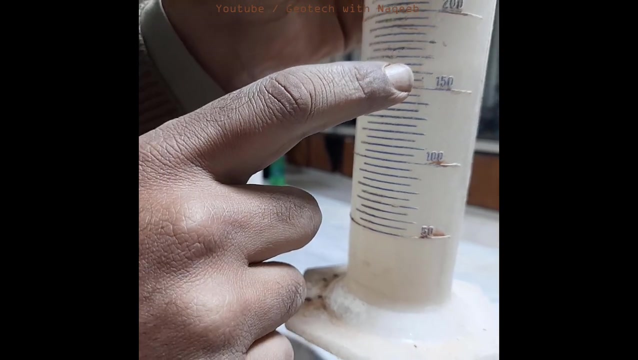 seven percent of 2355 gram. so the seven percent of 2355 gram is comes out to be 165 gram. so now, here you can see, we have 165 ml is equivalent to the 165 gram approximately. now we'll add this much amount of water into the soil. 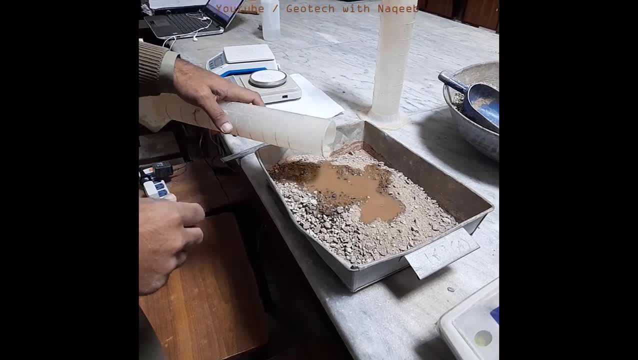 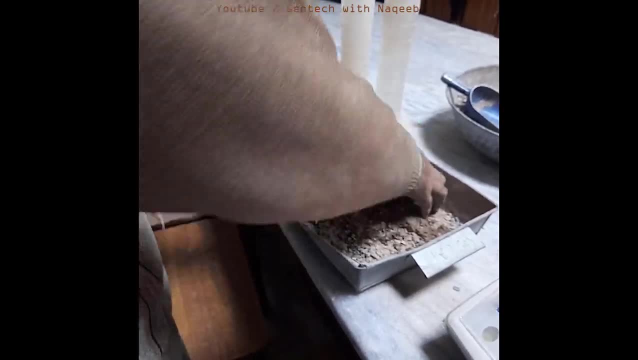 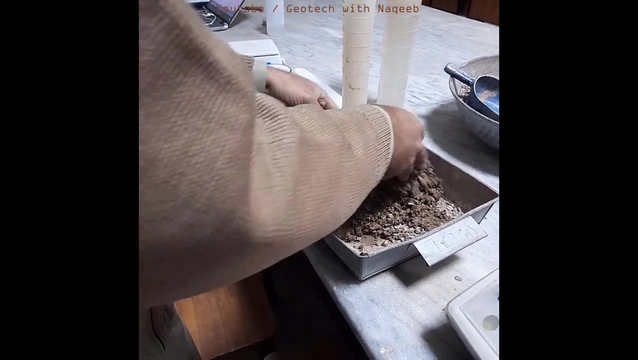 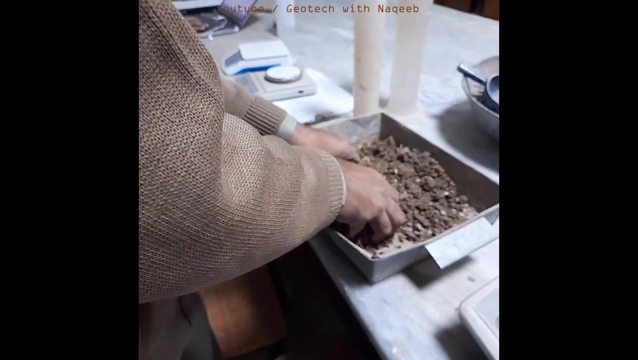 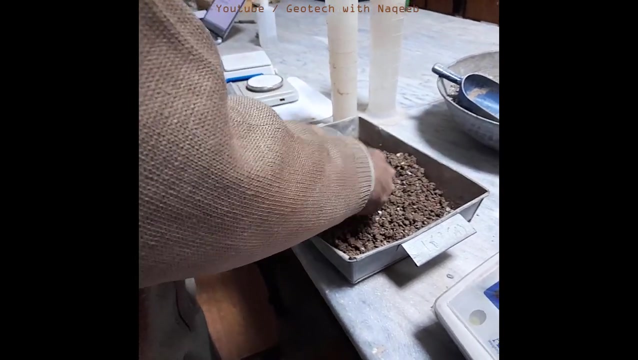 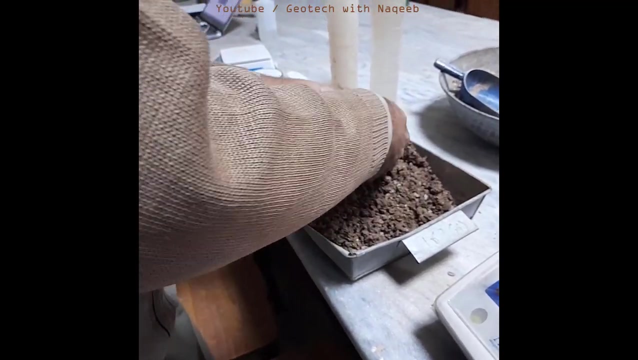 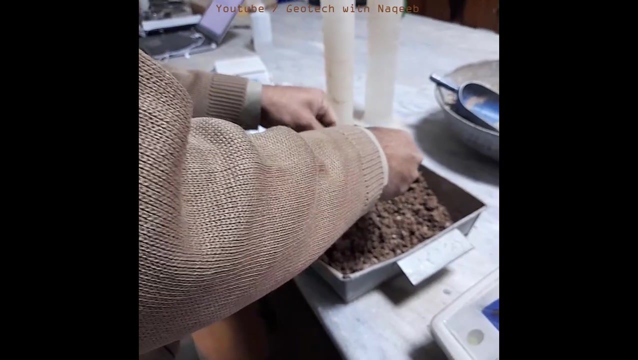 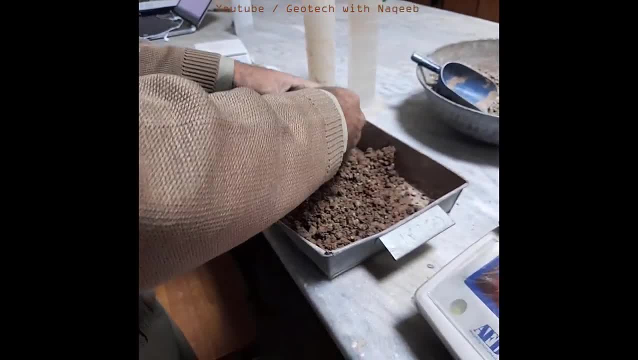 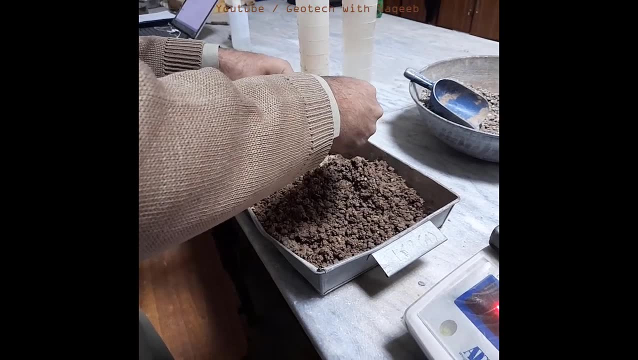 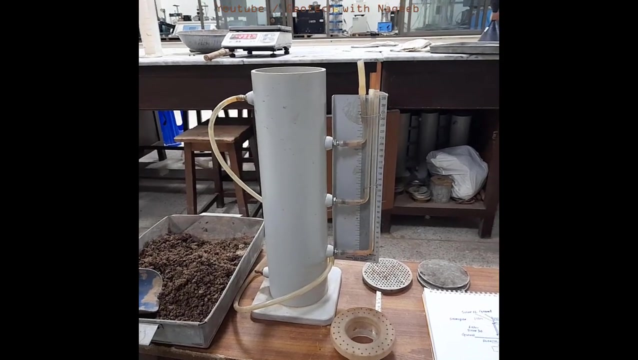 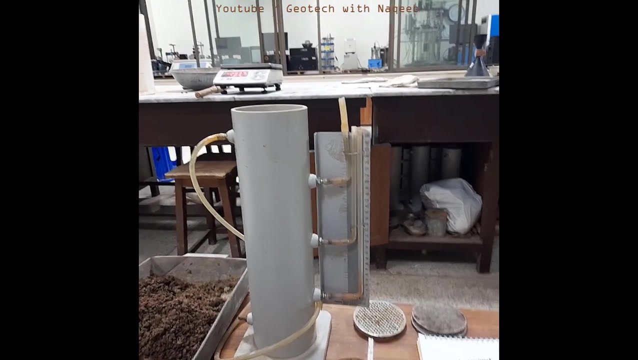 so these density and muscle content. so these density and muscle content, so these density and muscle content values can be dependent from proctor test. other ways these values can be dependent on site, but we need to understand that how we basically setup the assembly of the opportunities to perform test. so the preceding questions may require additional details from proctor test. so these density 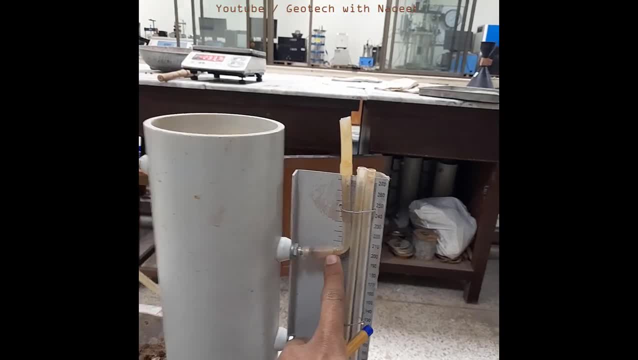 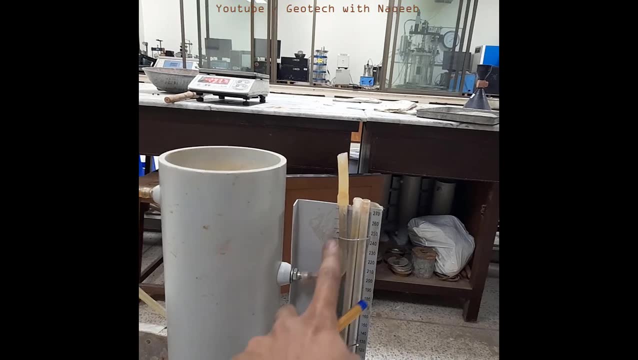 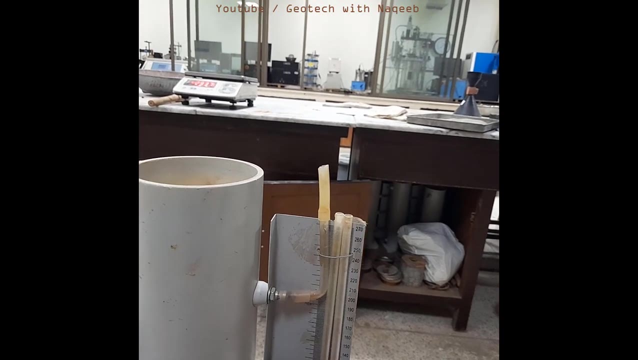 to know the these burets. first, the this buret is related to the constant head. so in this buret the head of the water is constant always. so that is why it is constant head test. now the second buret is related to the difference of the head. it tells us about the head difference in the water. now the 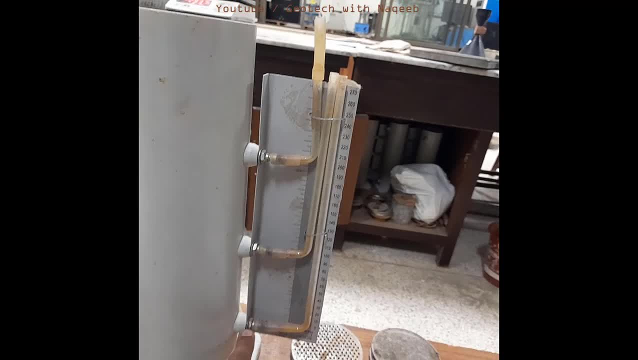 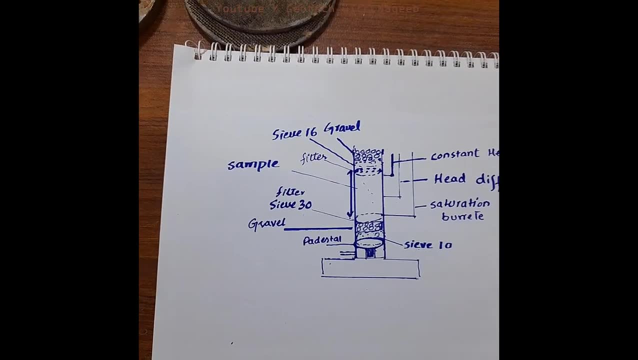 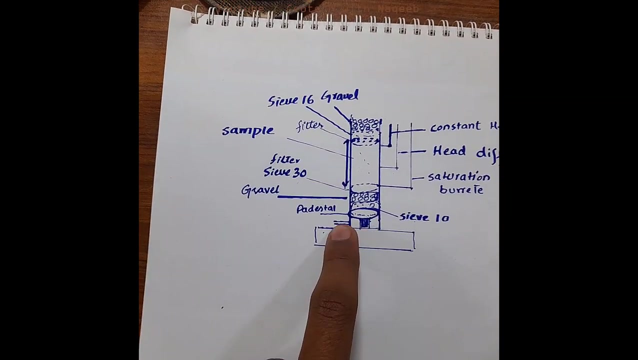 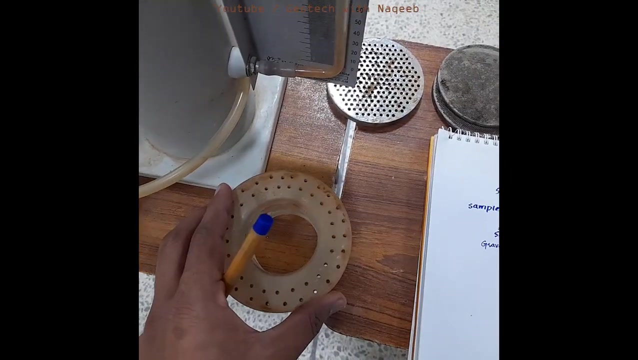 third buret is related to the saturation. so it tells us about the saturation. now, and to understand the assembly of this apparatus, that how we assemble the operators- here you can see the diagram. firstly will place the pedestal. you can see here. this pedestal will place in the bottom. 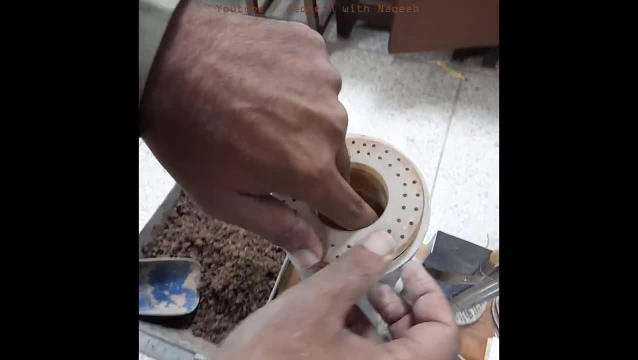 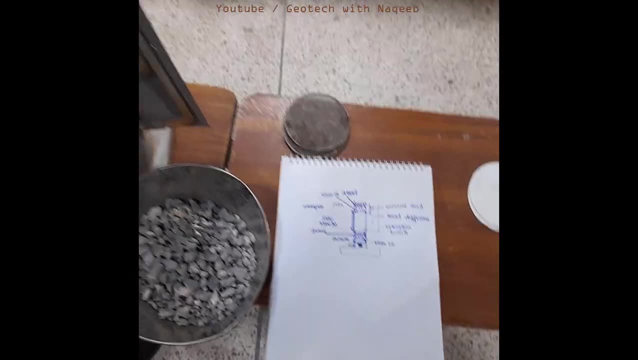 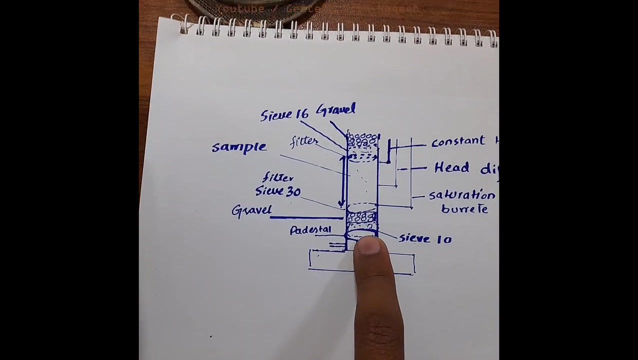 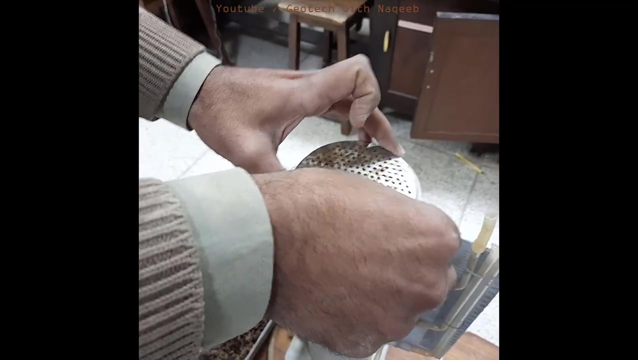 so now we'll place pedestal in the bottom of this mode. so after placing the pedestal in the mode now we'll place sieve number 10 over the pedestal you can see here. so now we'll place this sieve number 10. this is basically sieve number 10. opening of this mesh is basically see number 10. so we'll place the sieve number. 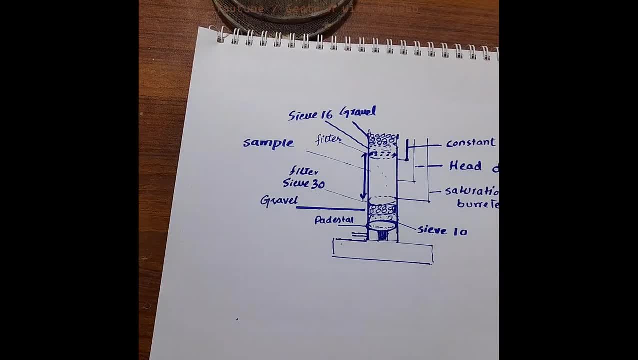 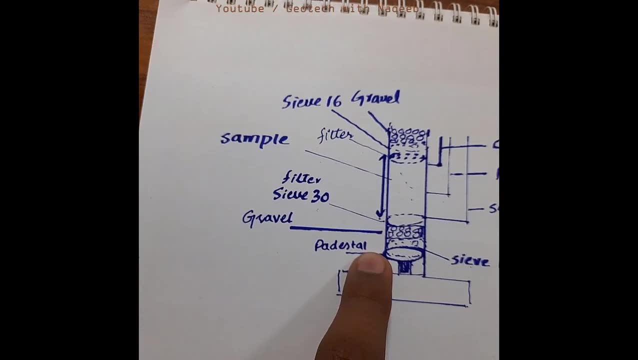 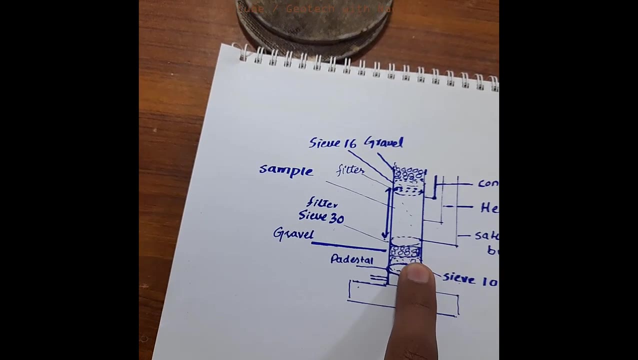 10 over the pedestal. now, in the next we'll place some gravels. you can see here gravel layer over this, so it will be up to the and this buret size to the saturation buret. so the thickness of this gravel layer is up to this saturation buret. 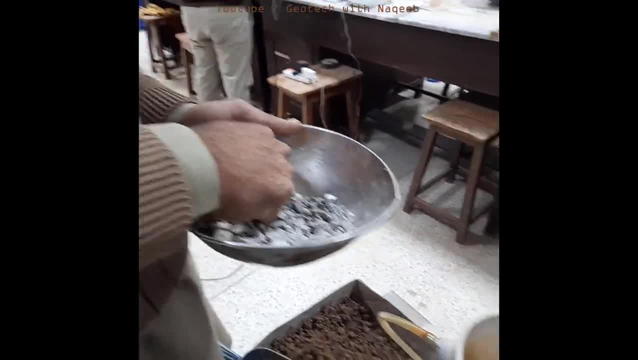 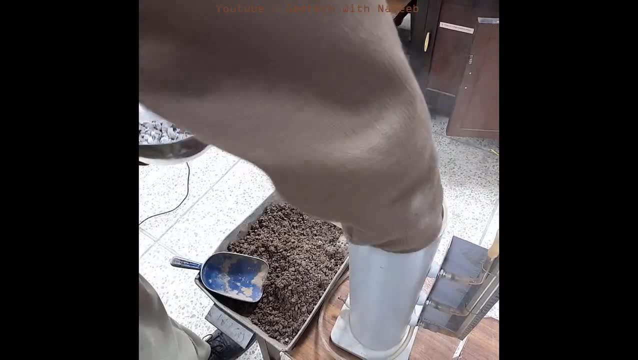 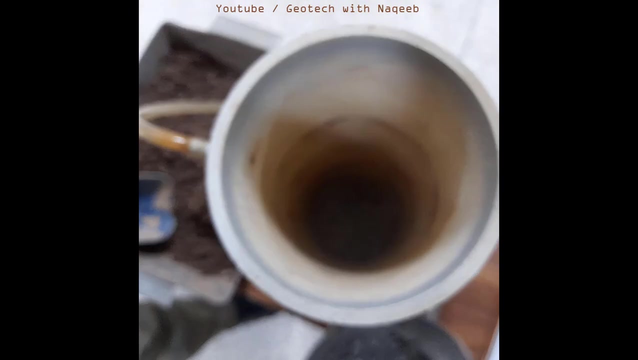 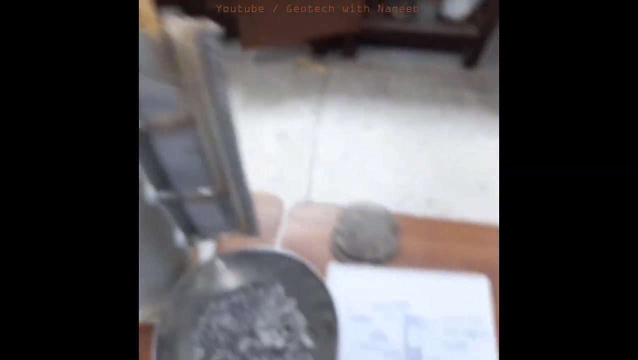 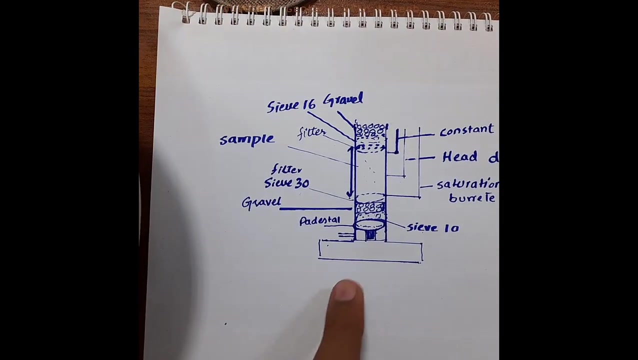 so now we'll have to visually inspect the level of the graph. now you can see the gravels have been placed in this mold up to the up to the saturation buret. now, as I told, next we'll we'll place sieve number 30 over this gravel and then 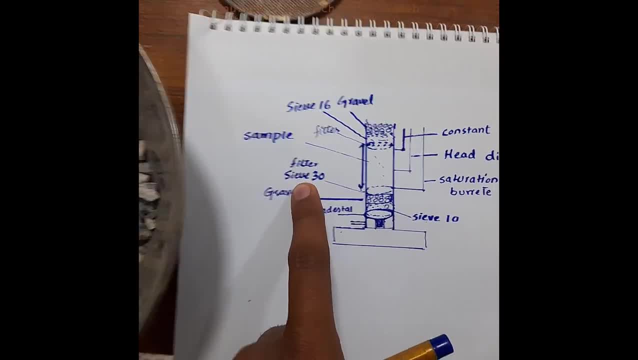 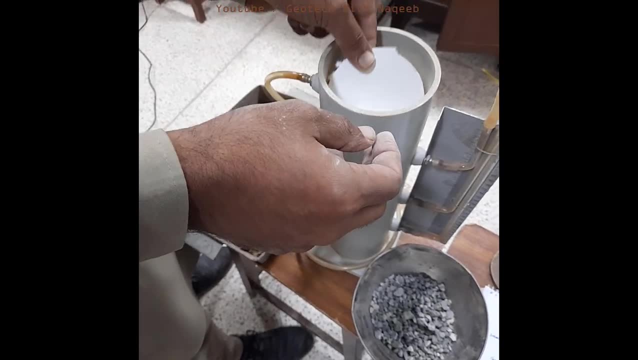 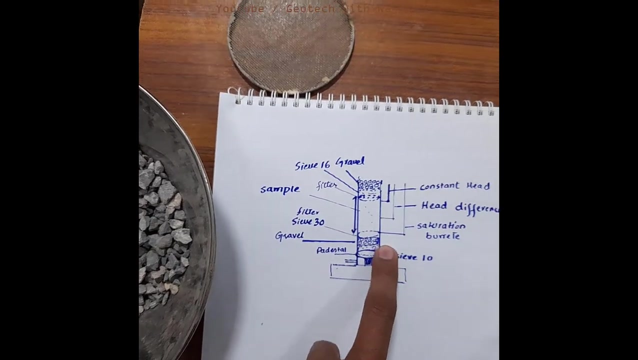 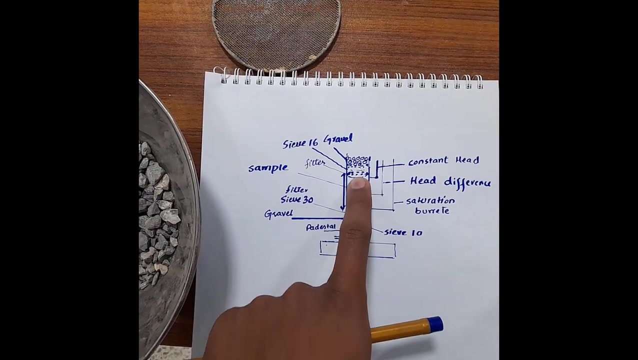 filter over this sieve number 30. so this is sieve number 30. and filter paper over sieve number 30. now, here you can see, this much height is filled up with the assembly apparatus. now we'll place the remolded soil sample, we'll place soil sample over here and we'll tamp it with the wooden rammer. 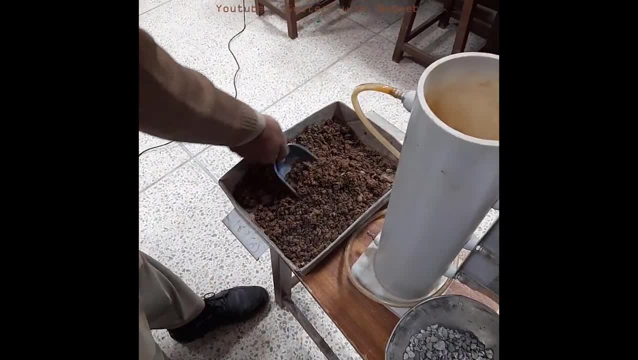 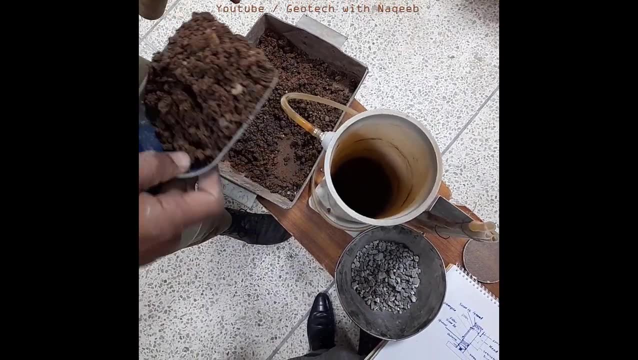 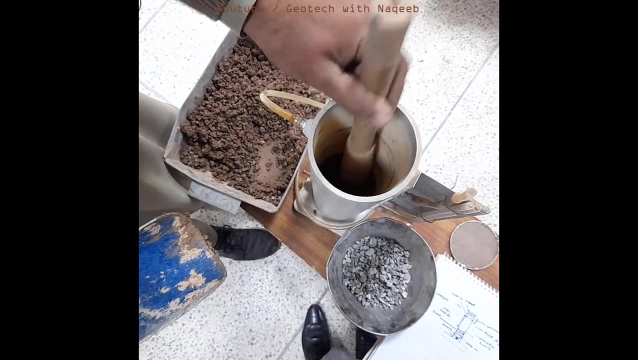 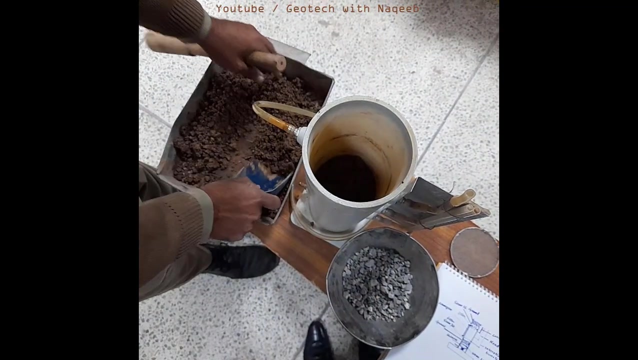 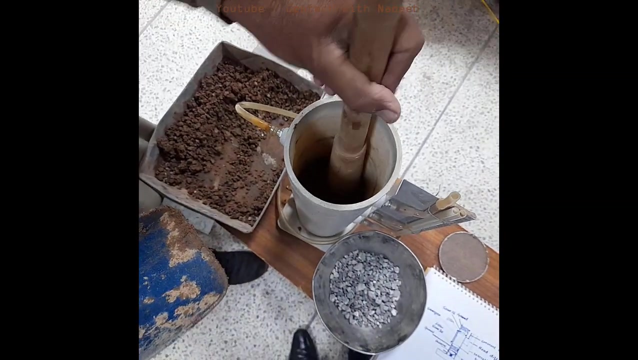 so now we'll place the soil sample. so we'll place the soil sample over here and we'll tamp it with the wooden rammer. remember potrze country, remember we have 20 centimeters and we have the volume calculated here. so, and to this you will need to fill desert JUICE. 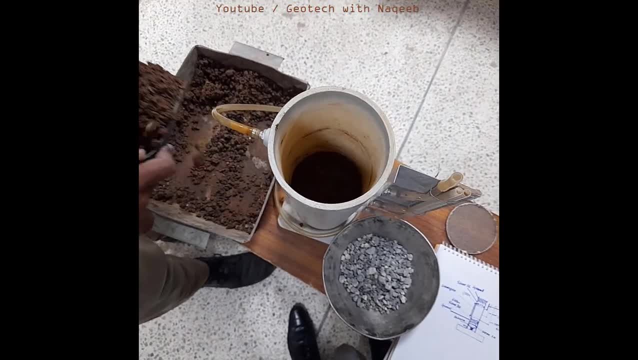 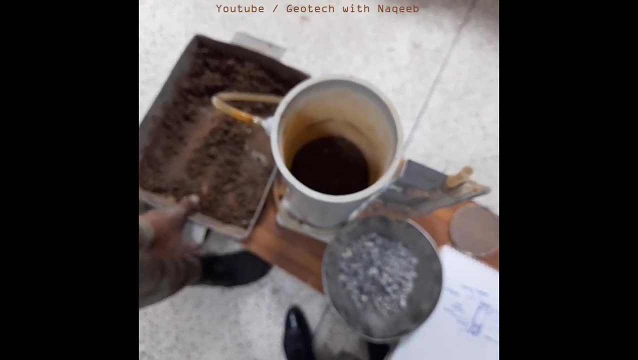 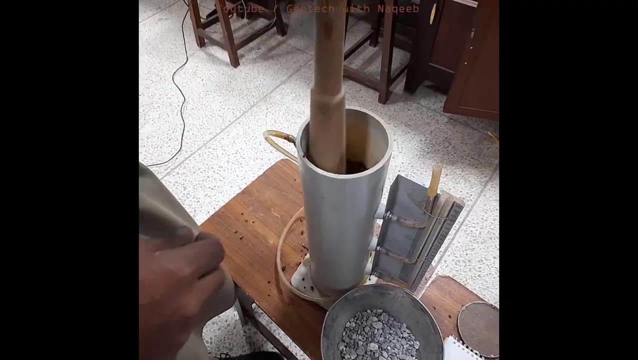 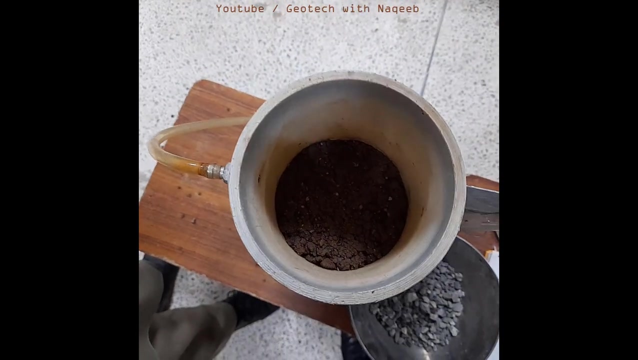 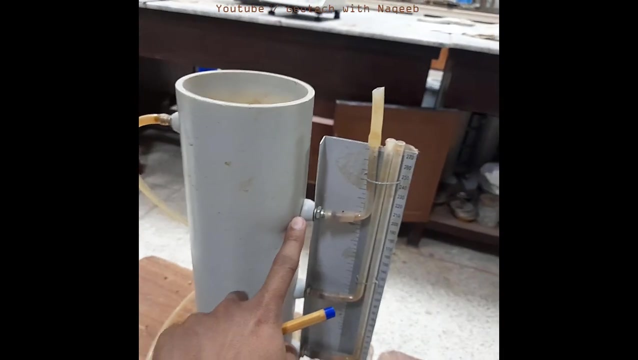 and to this you will need to fill desert JUICE and to this you will need to fill desert JUICE volume with this much amount of the soil. so now we have placed all the soil and in the mold and you can see the level. it is up to this, up to this burette, and as i earlier told that we have to restrict our soil. 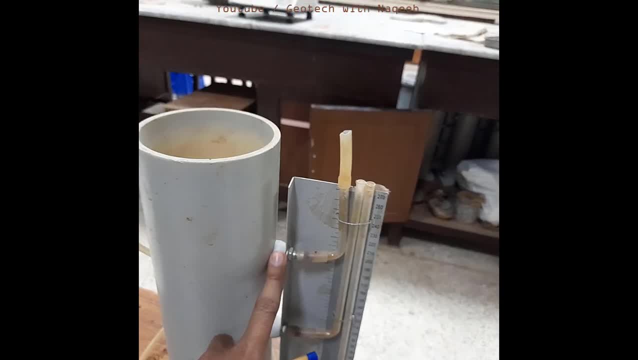 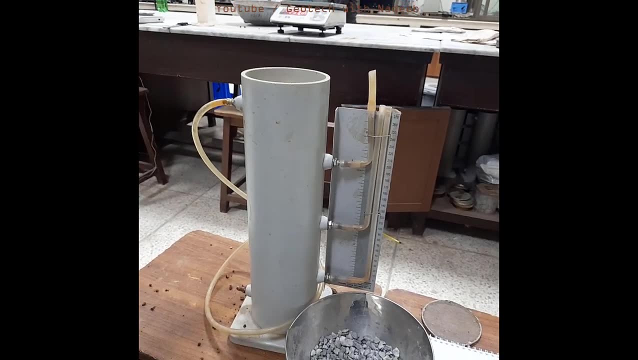 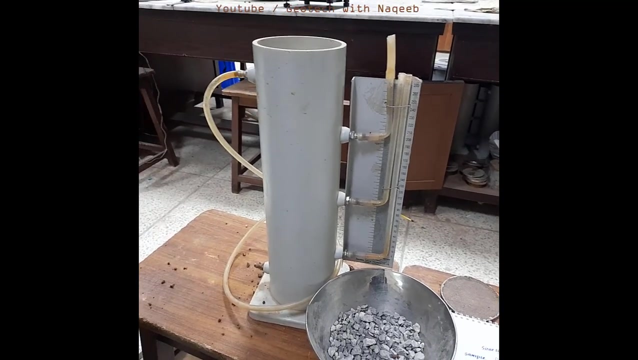 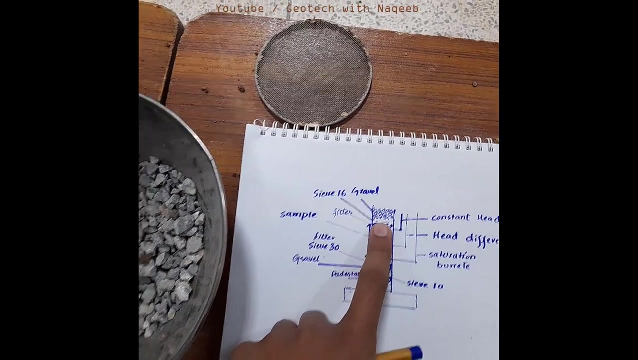 sample within this height. so this height is 20 centimeter and corresponding to this height we determine the volume. and that volume was used to determine the uh, the mass of soil required to fill that volume for remote soil sample calculation procedure. so now we'll place filter paper here. you can see in this diagram as well. we'll place filter paper over here. 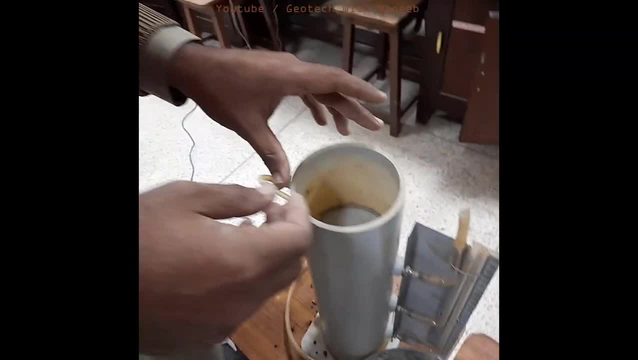 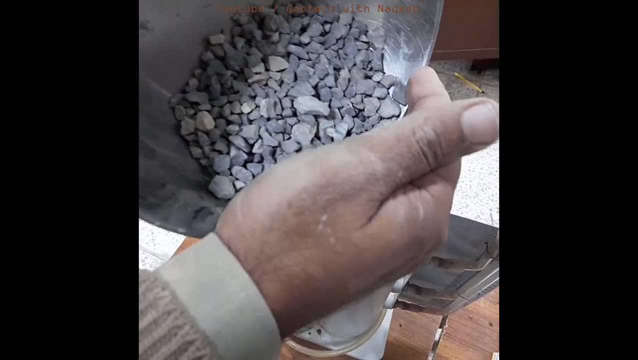 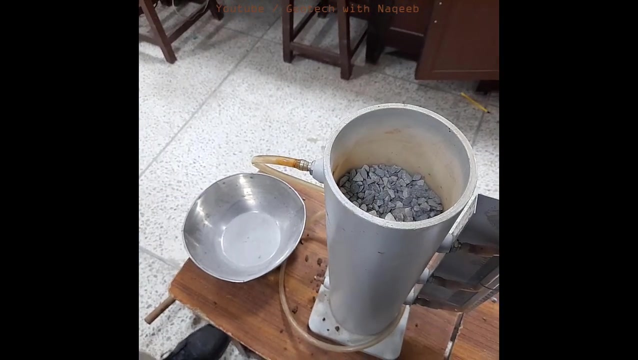 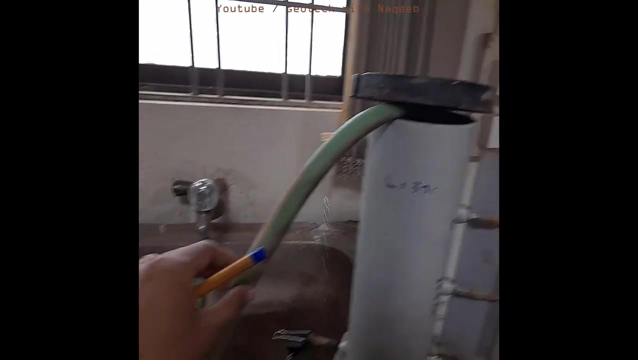 and now we'll place sieve number 16, sieve number 16, over there. now we'll place some amount of gravel. now our apparatus is ready to perform the test. so now, in the next step, we have to add the water in the soil sample. so we can use any way to add water in the soil sample. so we have 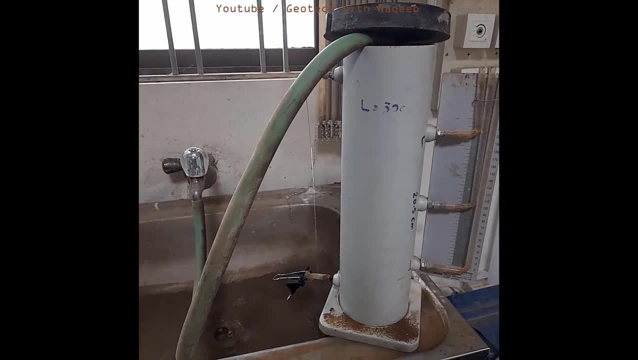 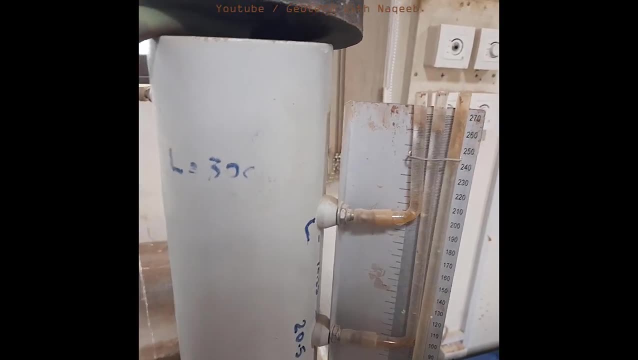 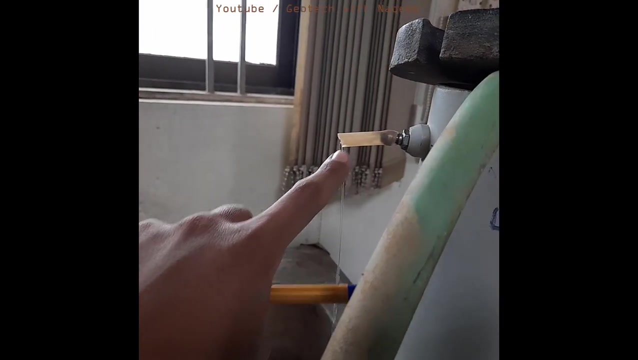 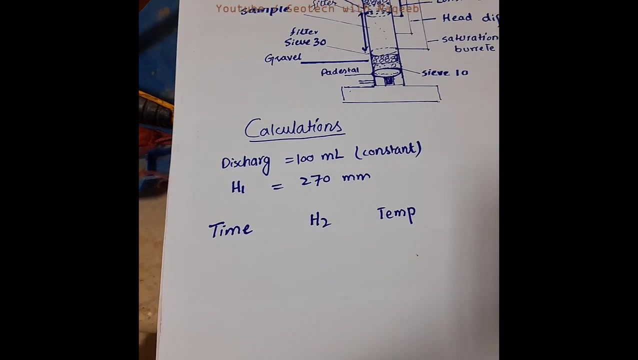 placed the mold over the sink to get the continuous water supply. and now here you can see when all the burettes are filled with the water, you can see the level of the water, and water starts overflowing from this, from here. it means our soil sample is now saturated. so now, uh, we'll, we'll, perform the test. 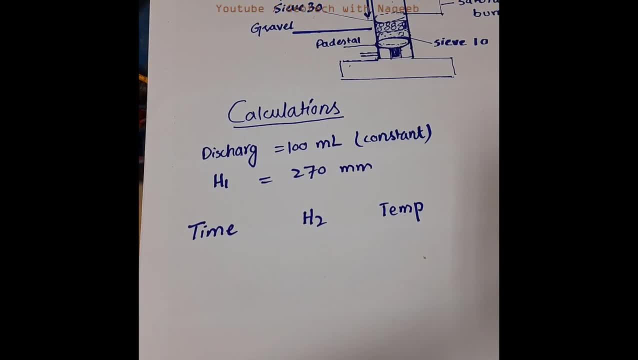 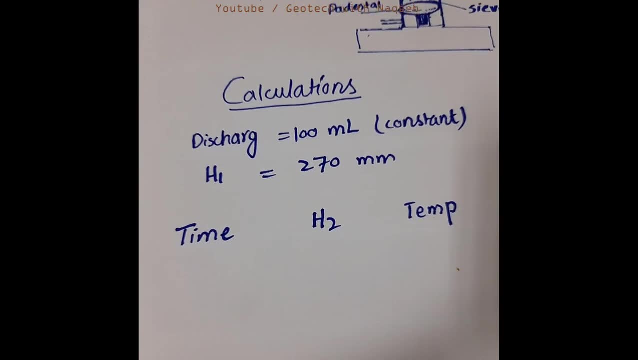 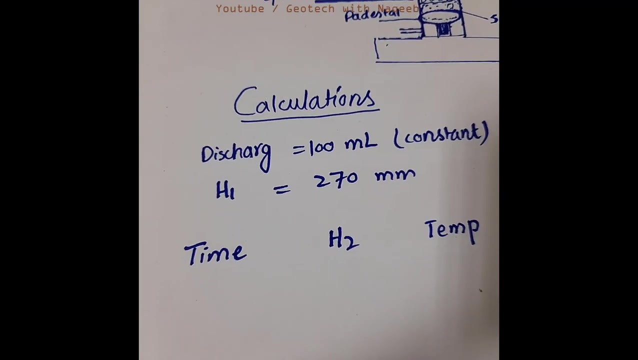 so to perform the test, we'll take the observations or readings. so, firstly, we have the discharge, 100 ml. that is constant. we can, we can fix the time as well, but in our case we have, uh, we have taken discharge as the constant value, that is, 100 ml, and we have had 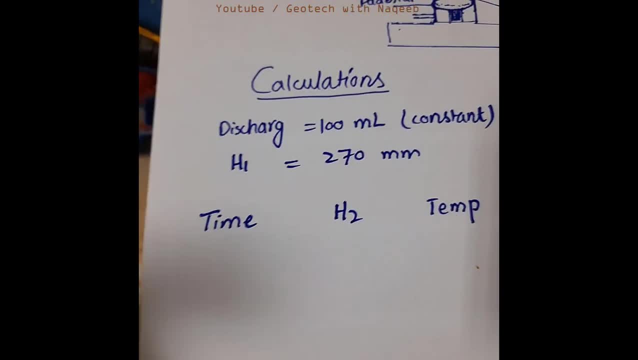 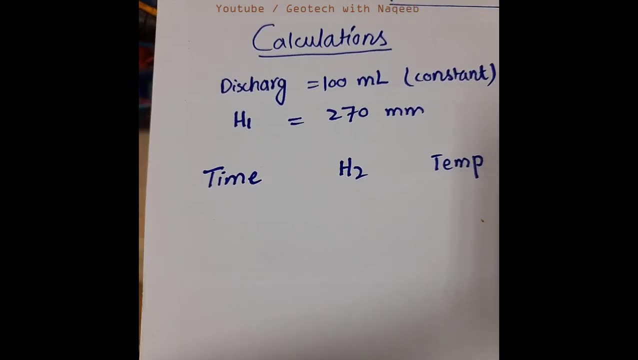 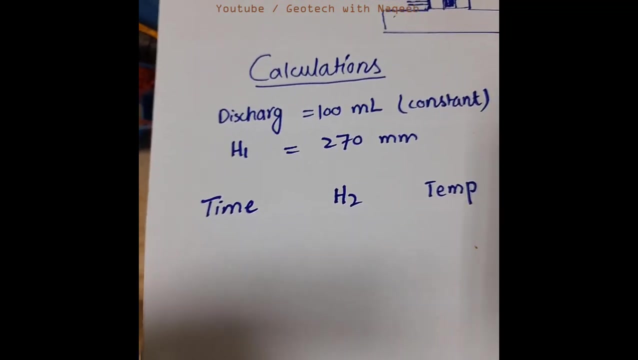 h1, that is 270 mm. that will be constant. that is why it is called constant head. so what we do, what we'll do is we'll have, we'll check the time and then uh time to fill the discharge of 100 ml and then we'll note it down- the h2 value and the corresponding temperature to perform the 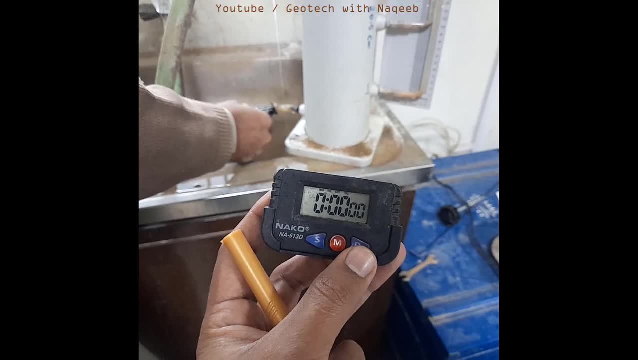 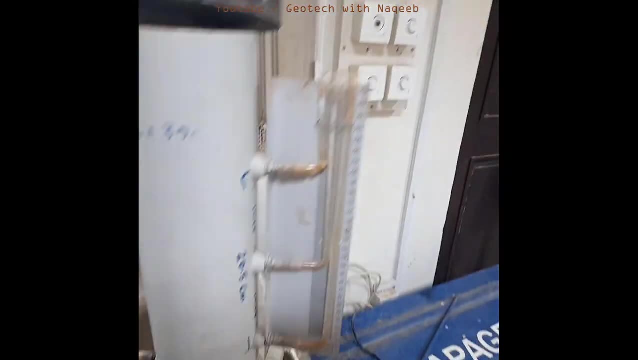 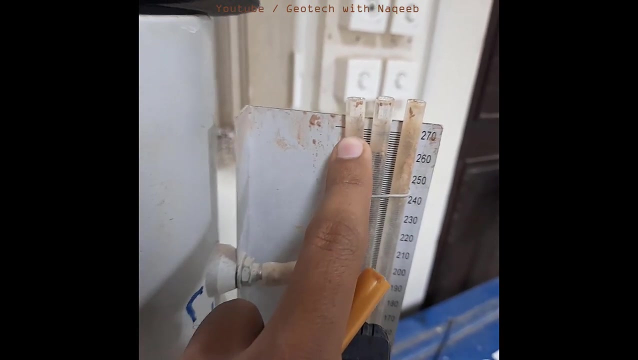 calculations. now we will perform the test. here we have the stopwatch and here from here we'll we'll collect the discharge from the mold and here you can see the h1 value. that is 270 mm. the head of the water in this burette will be constant, and that is 270 mm. here you can see. so now, 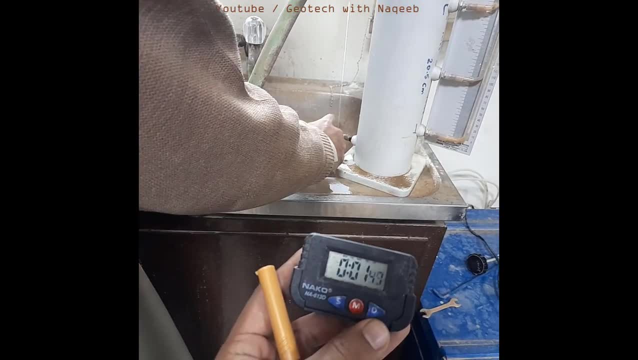 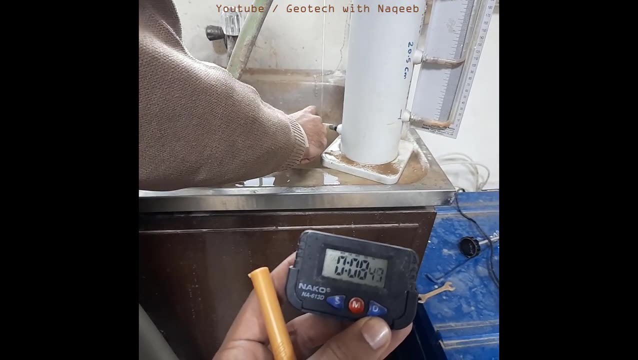 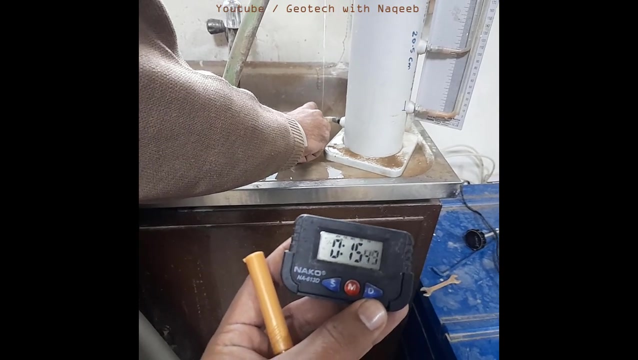 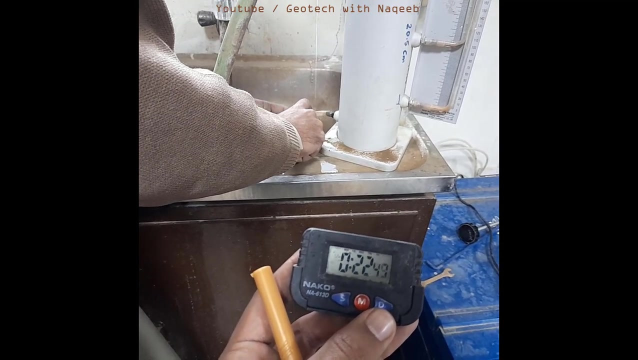 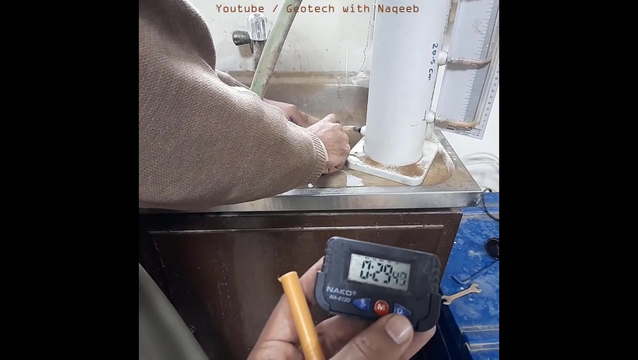 start, start. okay, now we'll note it down- the time required to have the discharge of 100 ml, so that will be used to perform the calculations to determine the hydraulic conductivity of this soil. so we actually require that time for time required to have the hundred ml. 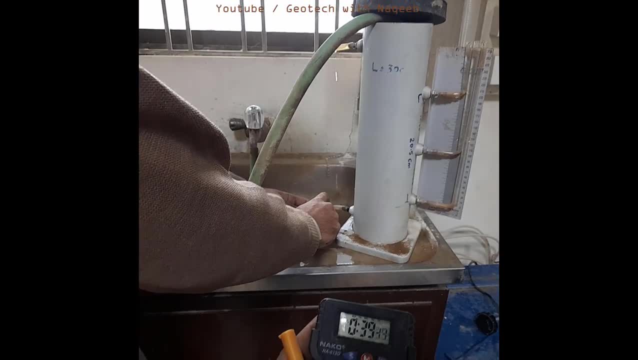 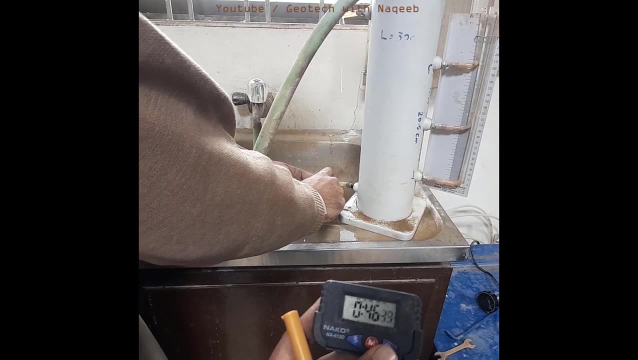 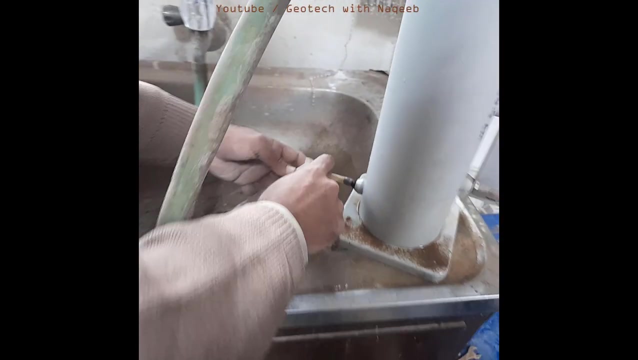 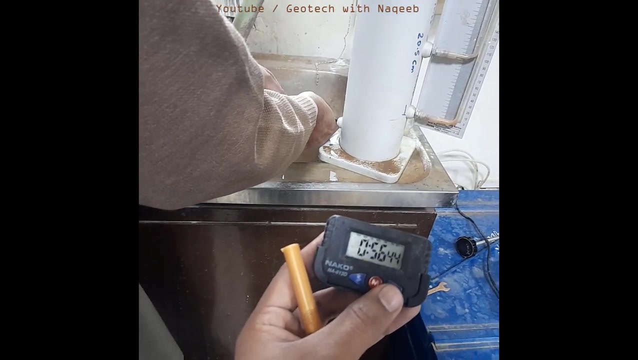 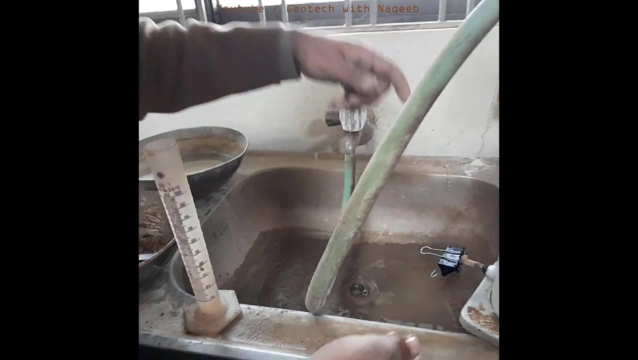 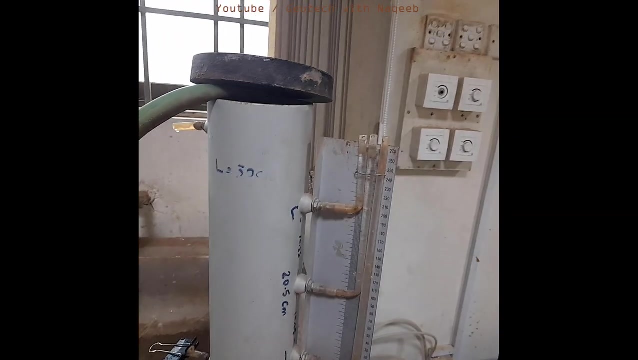 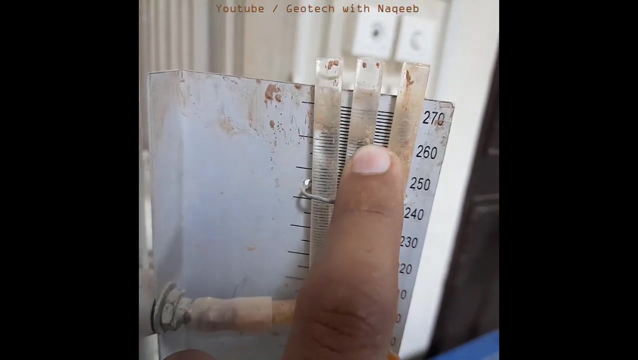 discharge from this soil sample. this is stop. so it means the 56 seconds. it took 56 seconds to fill the discharge of 100 ml. here you can see the 100 mm and how much the head difference is. you can see again. so the our second burette, the value you can see. the drop of head is basically. 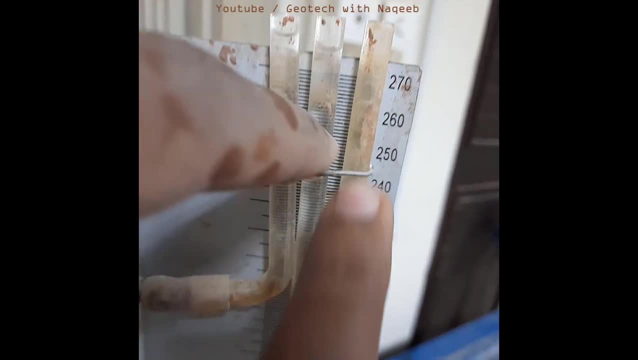 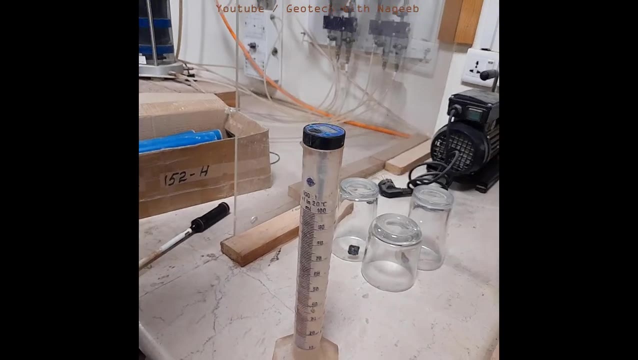 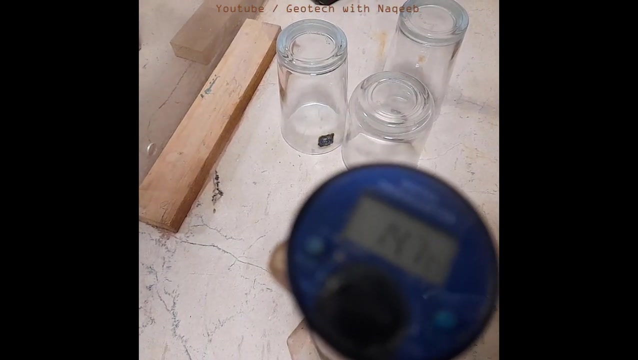 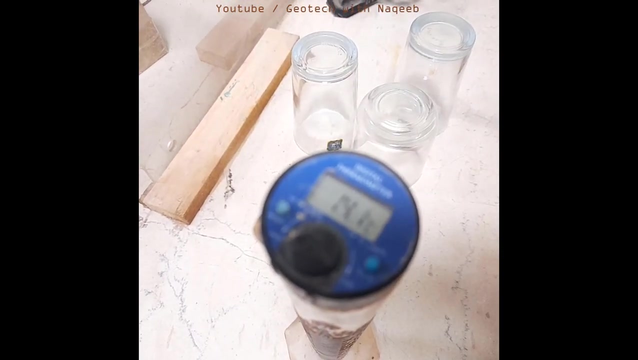 250 from this, from here, from, is now raising up again. now we'll check the temperature, because temperature affects the hydraulic conductivity and the temperature is when it will still be so the temperature is 14, almost 14 degrees. so now we'll perform the calculations. that how we 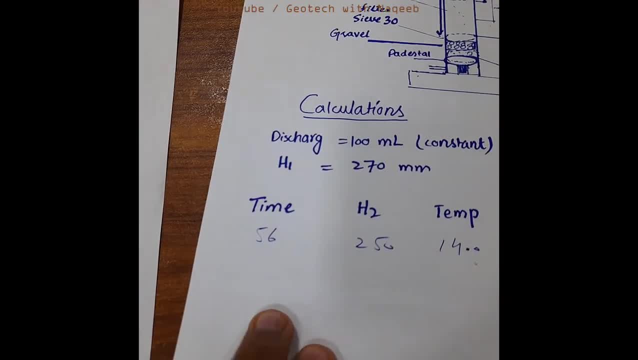 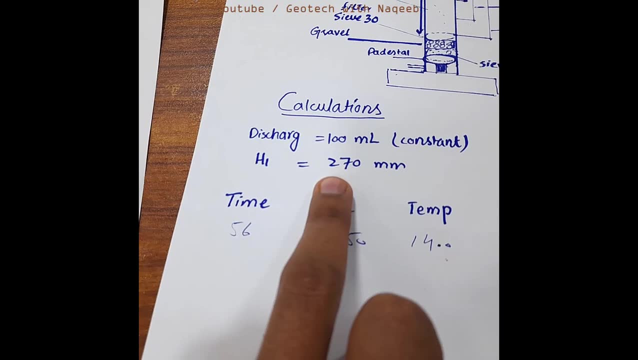 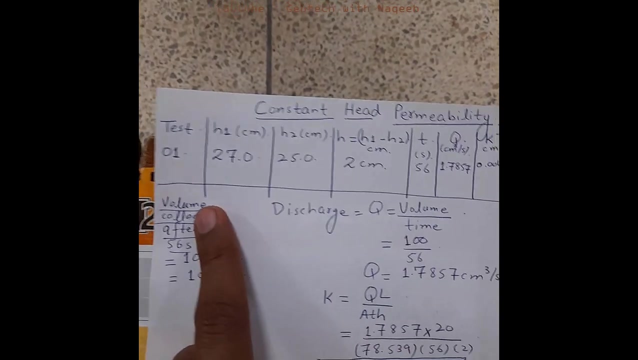 perform the calculations from the observations. we have the time, 56 seconds. we have h2 value head difference that is 250, the h1, that was constant, the value is 270 mm. and we have the temperature, that is 14 degree celsius. now let's see how we basically perform the calculations. here you can see the trial. we 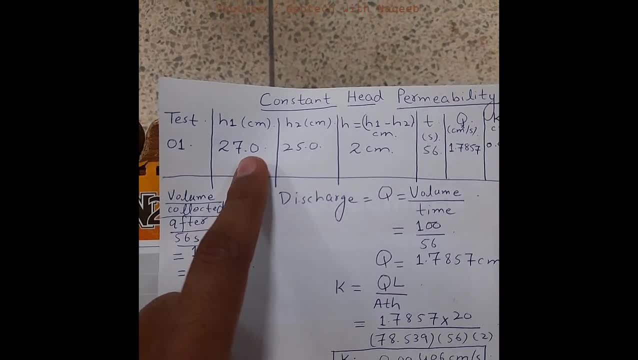 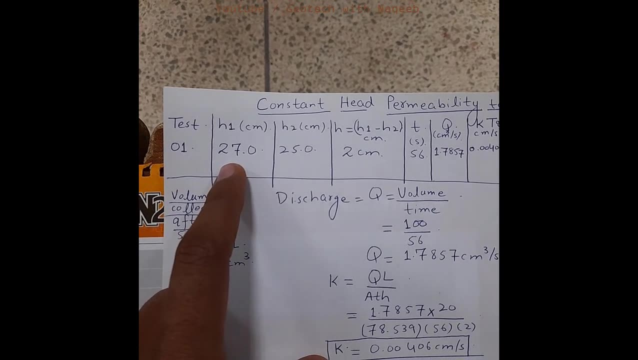 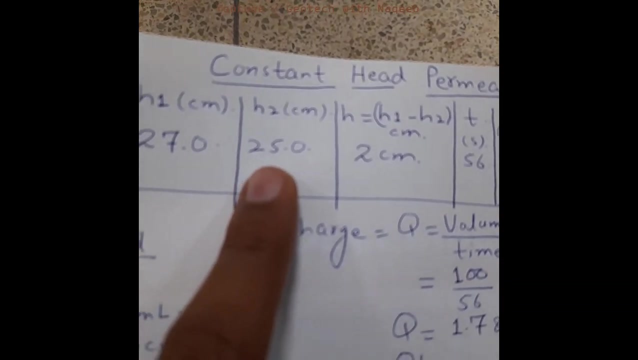 have performed the one trial. now we have h2 value that is in centimeters. 270 mm is the h1 value. if we convert this value in centimeters, it comes out to be 27. then we have h2 values. that was 250 mm and in centimeters this value will be 25.. now we need to find out the head. 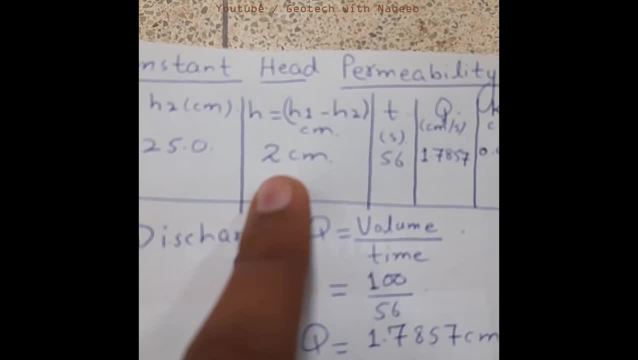 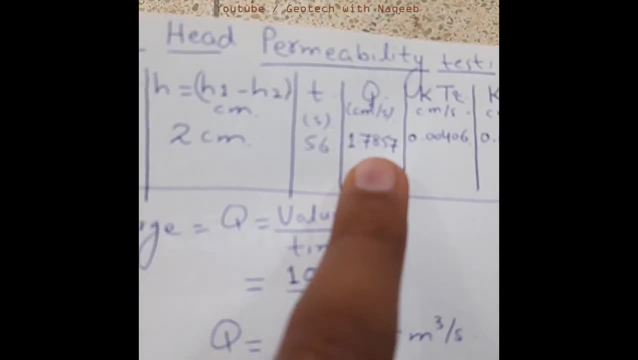 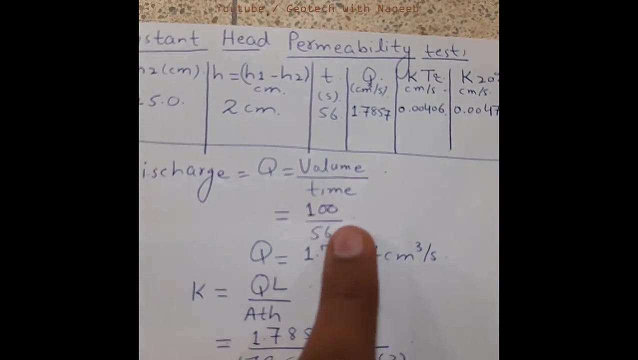 difference. so head difference is basically 20 mm, or we can say two centimeter, and the time was the 56 seconds. and now we'll have to calculate the discharge value. so how we can find out the discharge value. we have the volume, that is, 100 ml. the fixed value of the first discharge value is 12.5. mL and now we will have to calculate the discharge value. say, it is 10.5 mL, that is from the right side, and now we will have to calculate the discharge value. we have the volume in values. strength in our magic in this case May be 10.8. велises size for the primary and other values. consequently, 310 will be. in 12 is to 20 milliliters and 12 values for the secondary homes and indeed you can calculate back to the nucleus. so you need to calculate back thepie and if we construct that value says all this, we will get a massive value for the secondary. 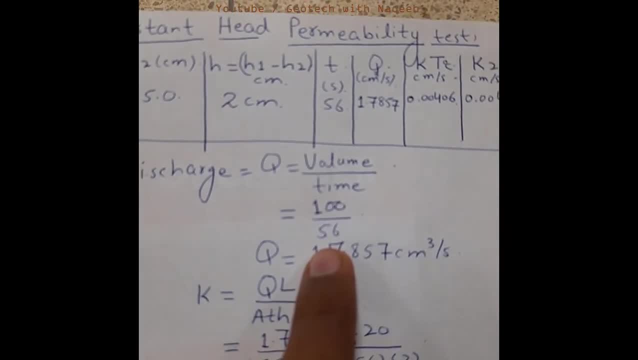 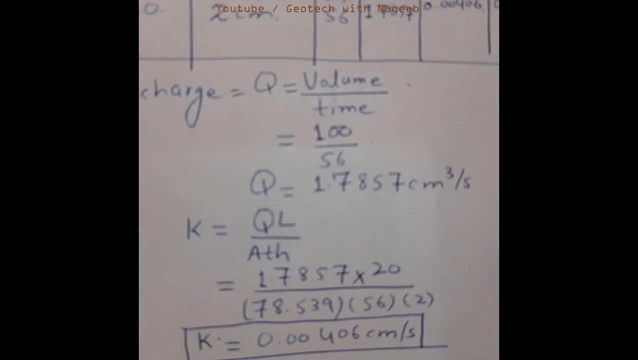 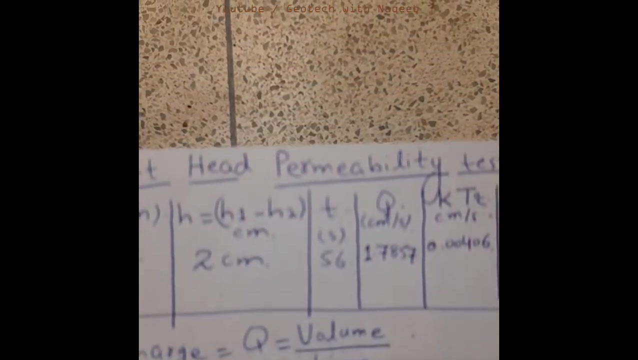 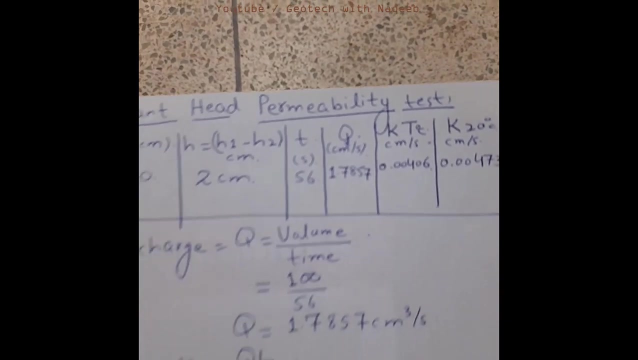 of the 100 ml value and we have the 56 seconds. so we need to find out the discharge value. that is, volume per unit time, and the discharge comes out to be 1.7857 cubic centimeter per second. now we need to find out the k value at temperature. that was the 14 degree celsius, so how we find. 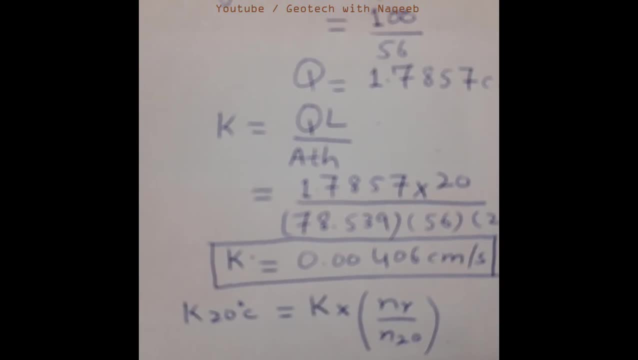 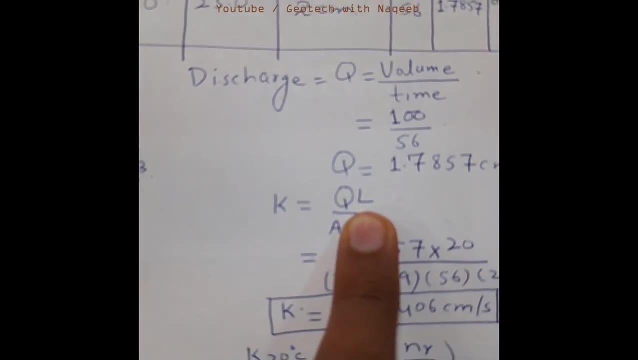 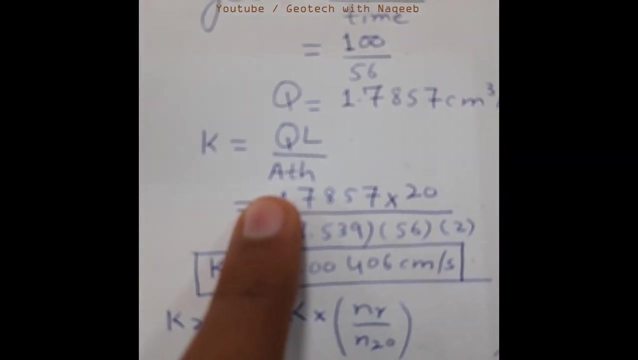 out the k value. the formula of k is q: l divided by a, t, h. l is the length of the soil sample. that was 20 centimeter, basically, and q we have calculated. now we have area that can be calculated from pi r scale, we have the time 60 second and we have the h value. that is head. 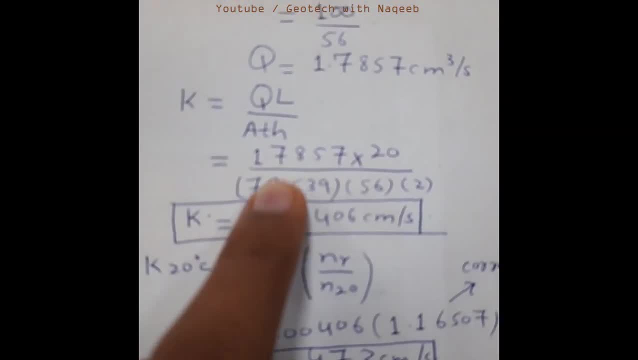 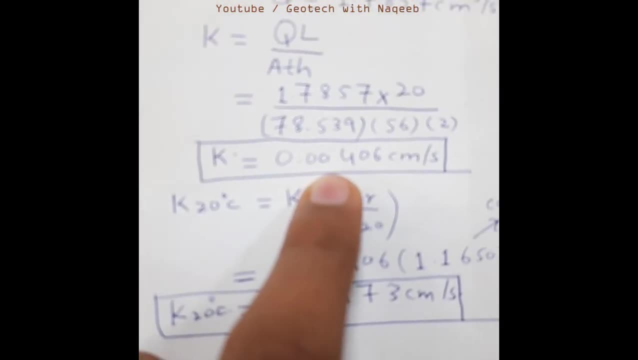 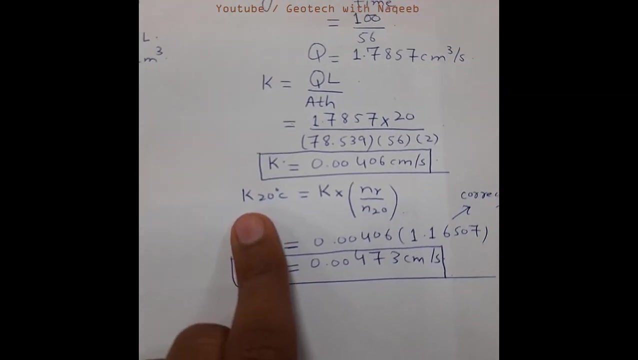 difference. that was 2 centimeter. so by putting the values in this formula and we can find out the k value, that is 0.00406 centimeter per second. but we need to find out the value at 20 degree celsius so to convert the value of hydraulic. 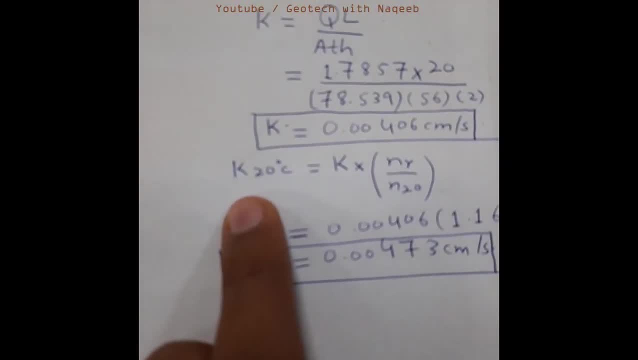 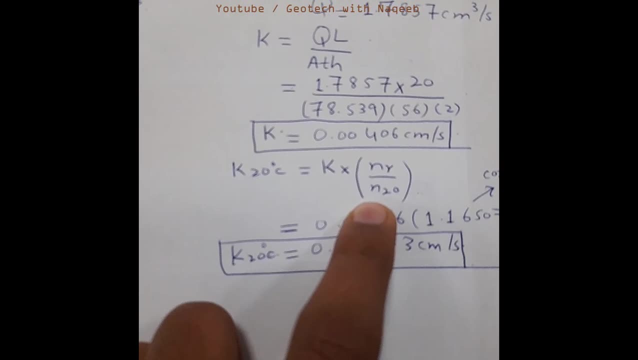 conductivity, or k value into 20 degree celsius, we need to apply correction. what we do? we multiply this k value with the correction that n gamma over n 20. that value can be extracted from the table that is given in the astm standard and we can find out the k value. that is 0.00406 centimeter per second. 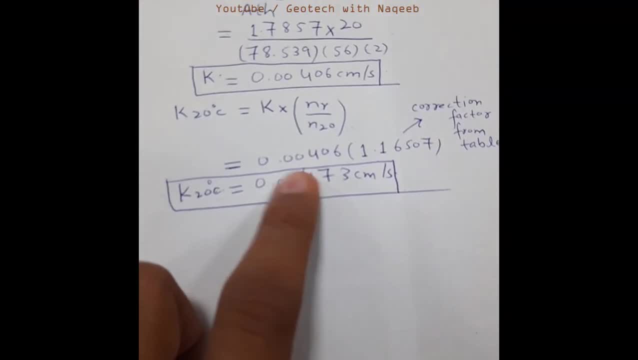 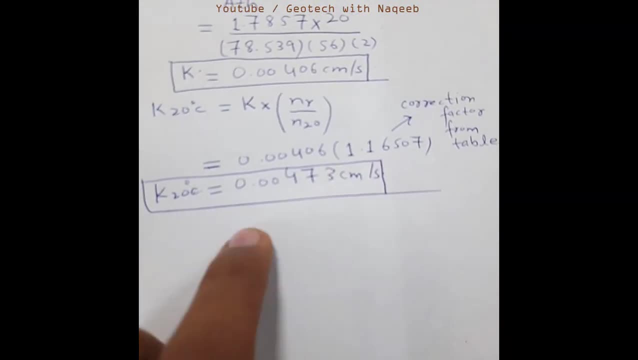 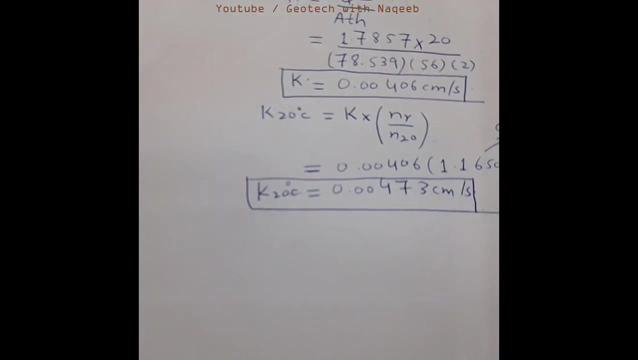 you can use that table and the value comes out to be 0.0046 multiplied by 1.165. that is basically the correction value and we the value comes out to be 0.00473 centimeter per second. so this is the value of hydraulic conductivity for constant head test. you.